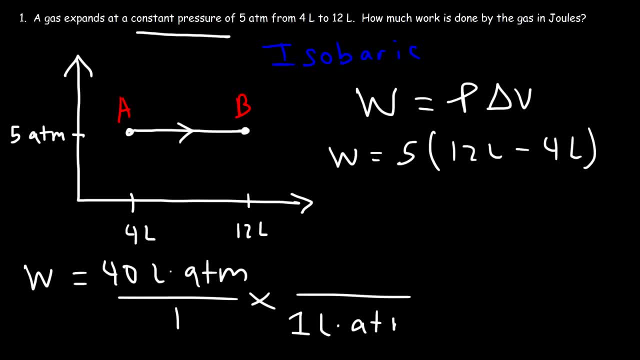 that to joules. So 1 liter times 1 atm is 101.3 joules. So that's the conversion factor that you need. So it's 40 times 101.3.. And so the final answer for this problem is 4,052.. 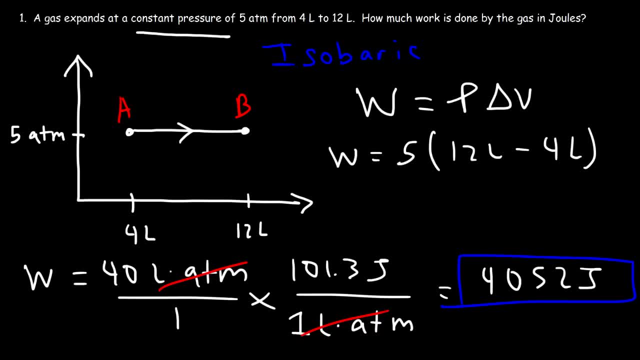 And that's it. Now. it's important to understand that the work done in a p-v diagram is the area under the curve, And so the area is left times width. In this case, the left represents the change in volume And the width is the pressure, And so that's what you can do. You. 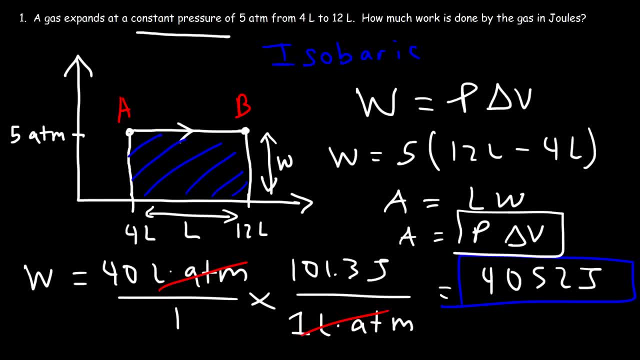 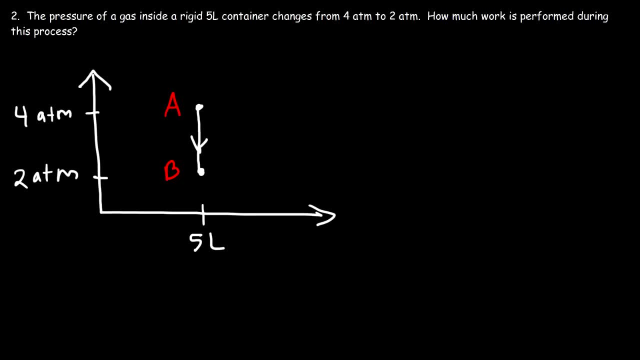 can get this equation. So the area is just the pressure times the change in volume. So make sure you understand that To calculate the work done from any p-v diagram, all you need to do is find the area under the curve Number two: The pressure of a gas inside a rigid 5 liter container changes from 4 atm. 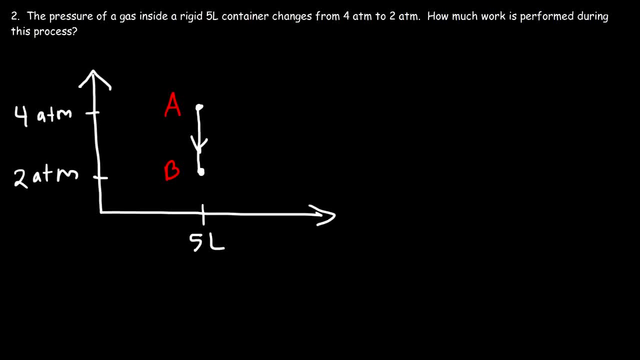 to 2 atm. So how much work is performed during this process? So notice that the volume of this rigid container is fixed, So the volume is constant. Therefore we have an isovolumetric, also known as an isochoric process. In this case the change in volume is zero. So notice that there's no shaded. 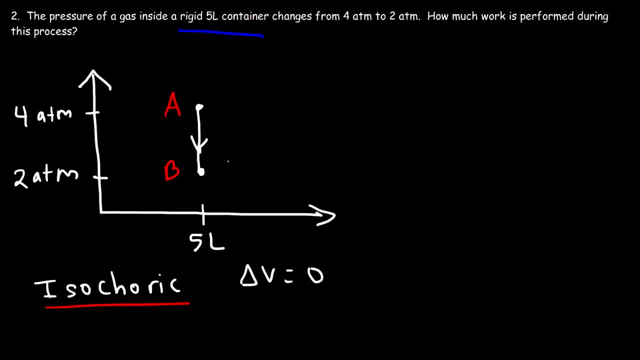 area or shaded region that you can draw in this diagram For an isochoric process, the work will always be equal to zero Because the change in volume is zero And work is really the integration of the pressure times, the change in volume. So if the change in 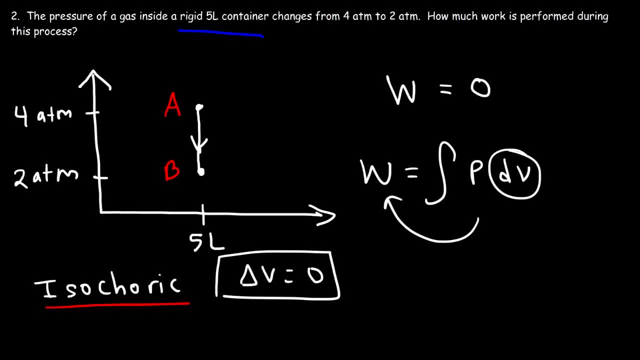 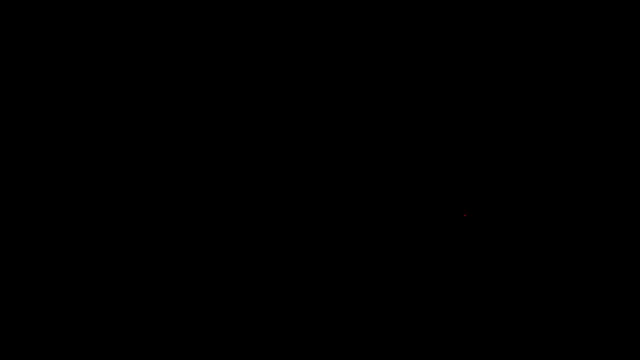 volume is zero, then the work is going to be zero. So this is always true for any isochoric process. W is always equal to zero. So keep that in mind. Number three: Five moles of nitrogen gas expands at a constant temperature of 400 Kelvin from 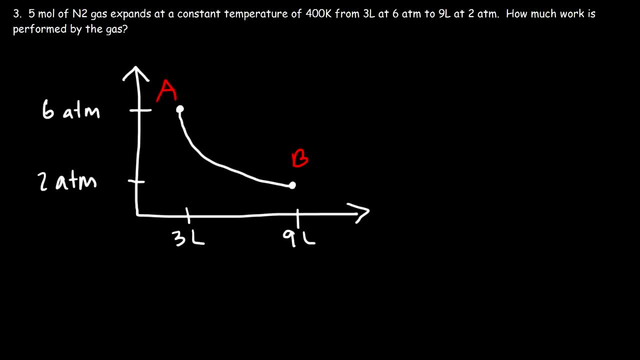 3 liters at 6 atm to 9 liters at 2 atm. How much work is performed during this process? Number two: The pressure of a gas inside a rigid 5 liter container changes from 4 atm to 0 atm. How much work is performed by the gas? 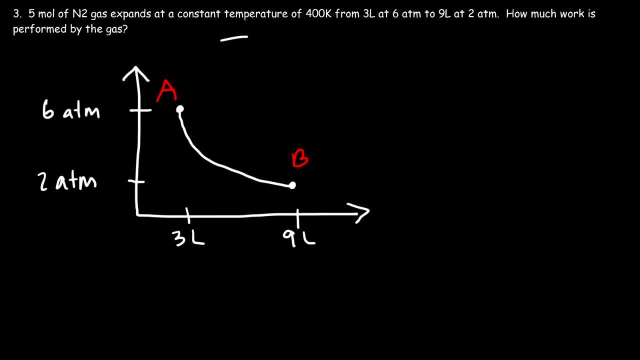 So this time the temperature is constant. So what we have is an isothermal process. The change in temperature is zero, And to calculate the work performed for an isothermal process, once again it's the area under the curve. Now it's not easy to calculate the. 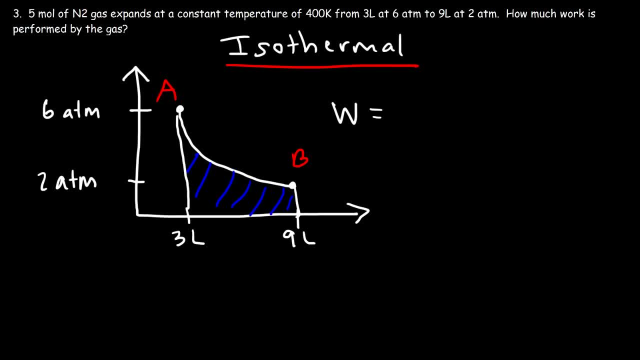 area under the curve in this example. Fortunately, there's a very simple way to calculate the formula that can help you to do so. It's nRT: natural log of the final volume divided by the initial volume. So n in this example is 5 moles, R is 8.3145 joules per mole per. 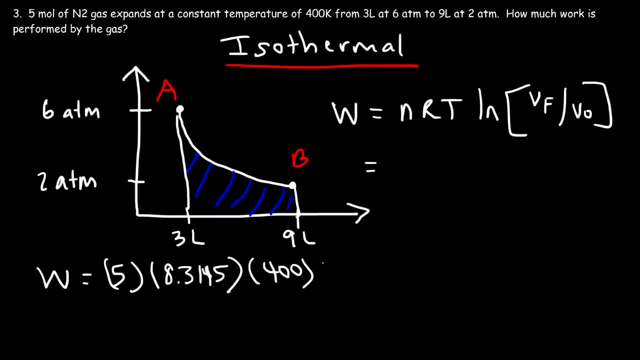 Kelvin And the temperature is 400 Kelvin. And then it's the natural log of the final volume, which is 9 liters divided by the initial volume of 3 liters. So it's going to be 5 times 8.3145 times 400 times the natural log of 3.. And 9 divided. 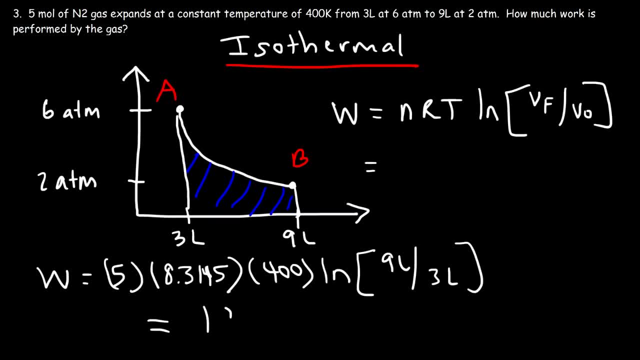 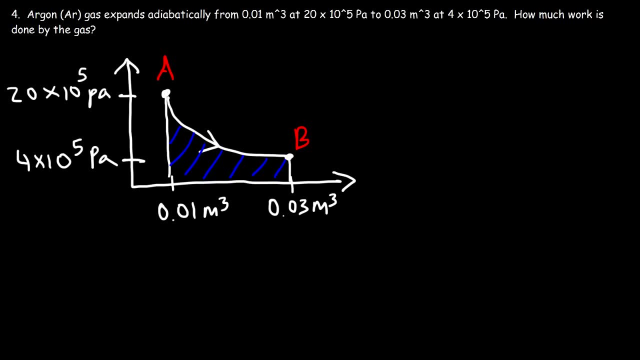 by 3 is 3.. And so W is going to be 18,269 joules. And so that's it for this problem. Number four: Argon gas expands adiabatically from 0.01 cubic meters at 20 times 10 to the. 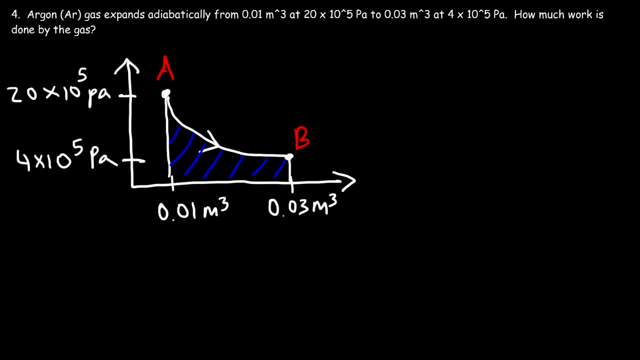 5 pascals to 0.03 cubic meters. at 4 times 10 to the 5 pascals, How much work is done by the gas For an adiabatic process? the heat transferred is 0. But we don't have to. 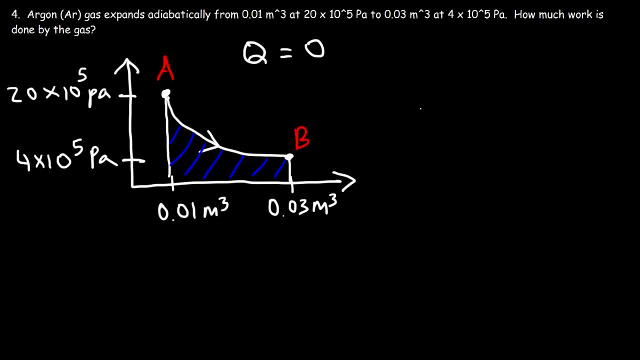 worry about that. in this example, To calculate the work, the formula that we need is negative Cv over R times the final pressure multiplied by the final volume minus the initial pressure times the initial volume. Now we have a monoatomic gas, And Cv for a monoatomic gas is 3 over 2 R, And so if we 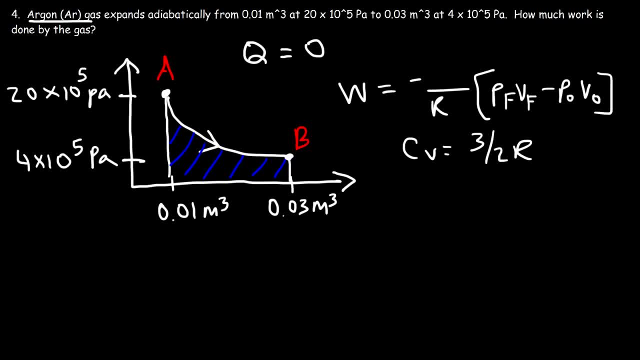 replace Cv with 3 over 2 R, we could cancel R. So for this particular example, W is going to be negative 3 over 2 R times the product of the pressure and volume minus the initial pressure and volume. So that's going to be negative 3 over 2 times a point. Well, that R should not be there. 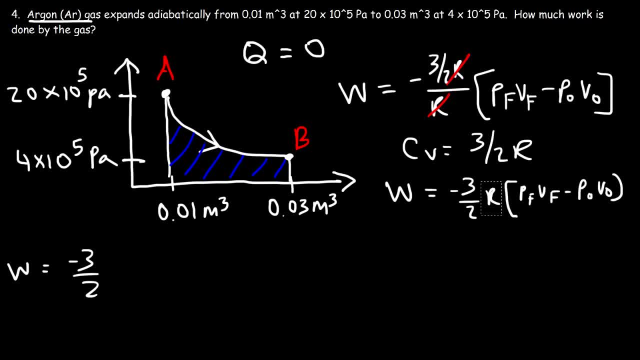 anymore. I don't know why. I wrote it again. So it's negative 3 over 2 times the final pressure which is at point B, That's 4 times 10 to the 5 multiplied by the final volume of 0.03 cubic meters. 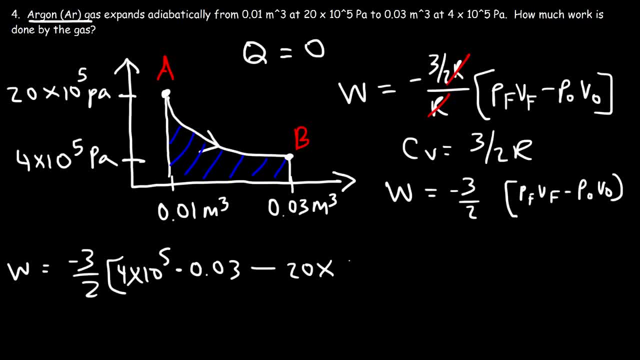 And then at point A, the initial pressure is 20 times 10 to the 5. And the initial volume is 0.01 cubic meters. So go ahead and type that in. I'm going to do it one step at a time, So first 4 times. 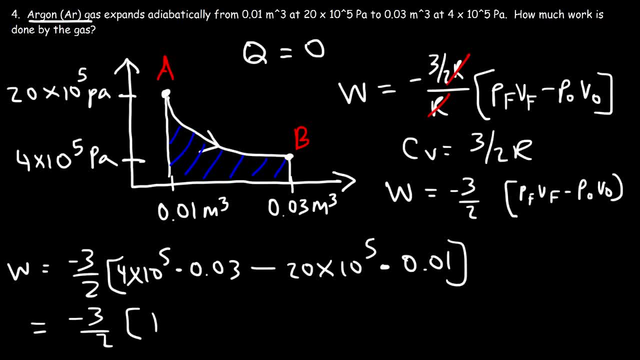 10 to the 5 times 0.03, that's 12,000.. And then 20 times 10 to the 5 times 0.01 is 20,000.. So 12,000 times 0.03 is 0.03.. 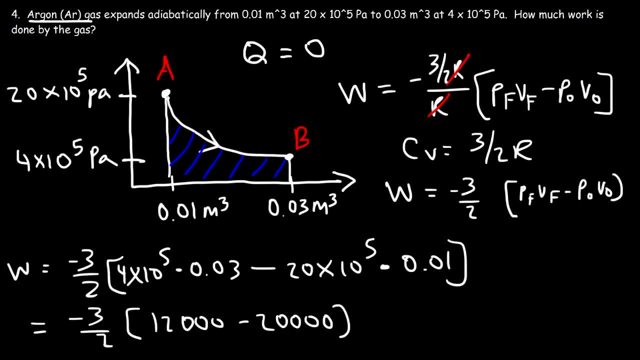 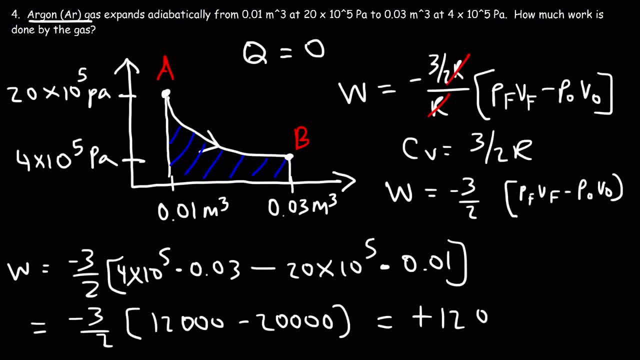 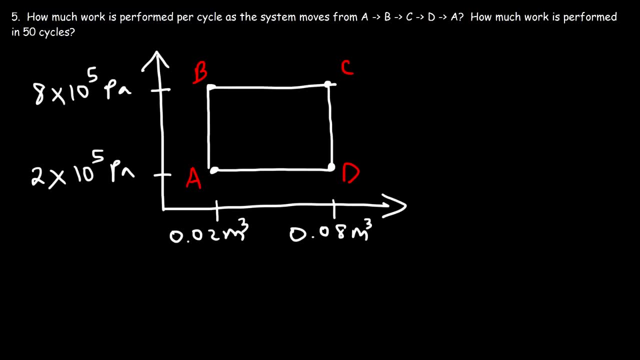 This is equal to a positive 12,000 joules And the work should be positive for any type of expansion process. So that's it for this problem. Number 5, how much work is performed per cycle as the system moves from A to B to C to D? 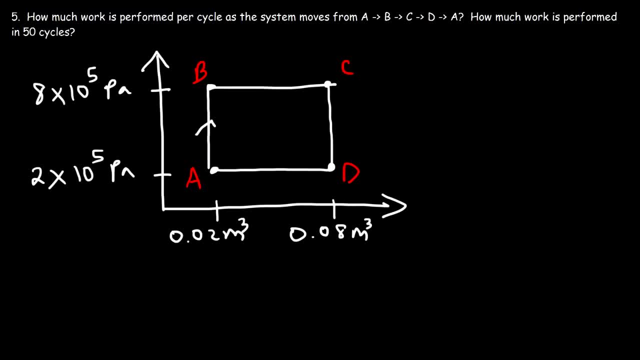 to A, So from A to B, It's going that direction, and then B to C, C to D, D to A. Now, to calculate the work perform it's simply the area that's enclosed by the PV diagram, especially if you have a cyclic. 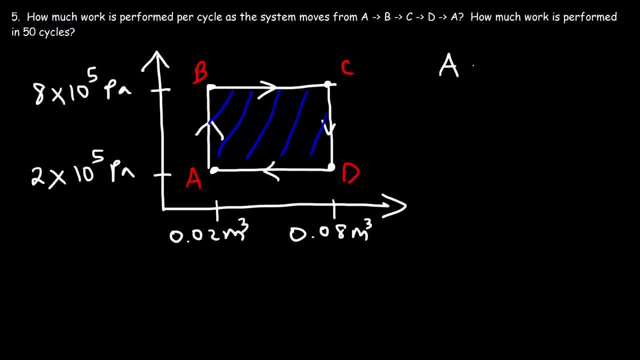 process. So the area is simply left times width. In this case, the left is basically the change in volume and the width is the change in pressure. So you can say it's delta P times delta V for this example. So the difference in pressure. 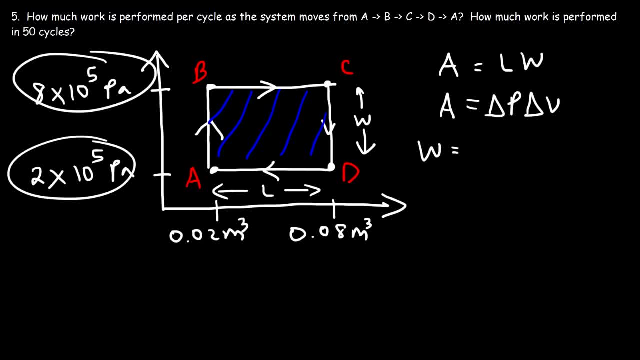 8 times 10 to the 5 minus 2 times 10 to the 5, that's the difference of 6 times 10 to the 5 pascals And the change in volume: 0.08 minus 0.02, that's 0.06 cubic meters. So 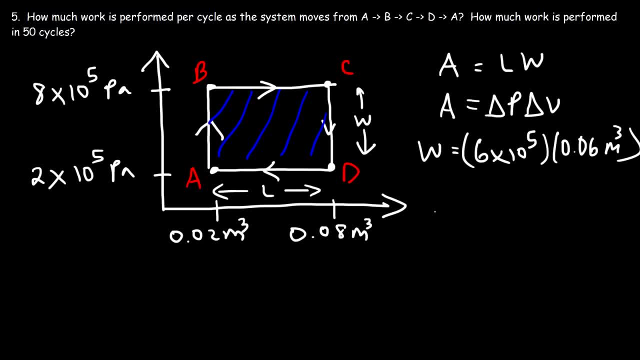 6 times 10 to the 5 times 0.06.. And so the answer is 36,000 joules. Now should this answer be positive or should it be negative? It has to do with the direction of rotation. Notice that the system is. 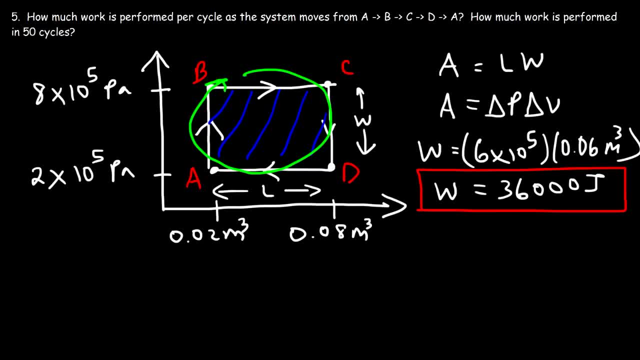 moving in the clockwise direction. So if it's moving in the clockwise direction, the work performed per cycle is positive. If it's moving in a counterclockwise direction. so let's say if it's going in this direction, the work performed per 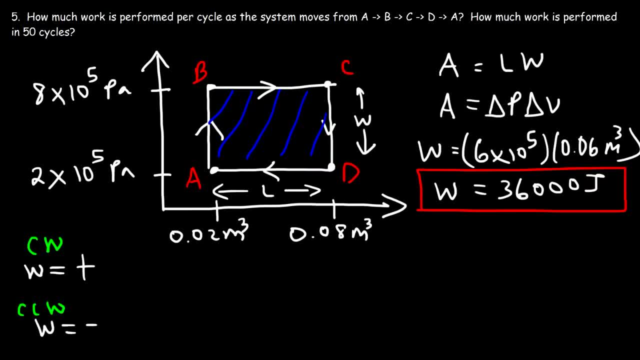 cycle will be negative. So for this example, it should be positive, since it's moving clockwise. Now we're going to confirm this answer by calculating the work for every step. So what's the work performed? going from A to B? From A to B? 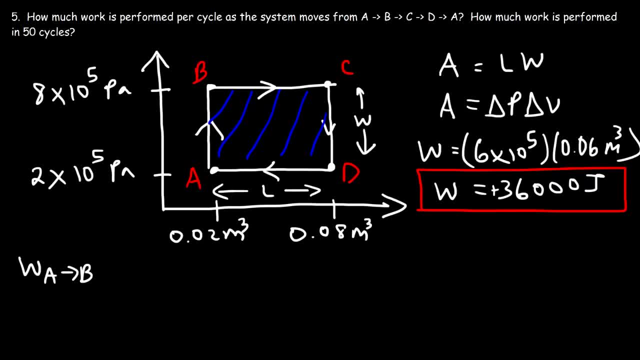 we have an isochromatic chord process. The volume is constant. It's 0.02.. It doesn't change, So it's 0. going from A to B and also going from C to D. whenever you have a vertical line, the 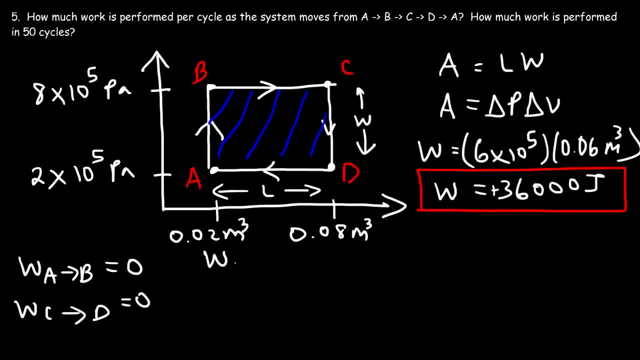 work is going to be 0.. Now, from B to C, we have an isobaric process because the pressure is constant, And so we could use this formula: It's going to be P times delta V, So the pressure is 8 times 10 to the 5.. 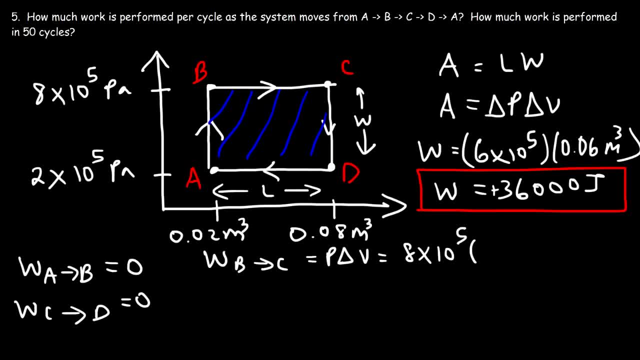 And as we go from B to C, the final volume is 0.08.. The initial volume is 0.02.. So this is going to be positive. 0.08 minus 0.02 is 0.06 times 8 times 10 to the 5.. 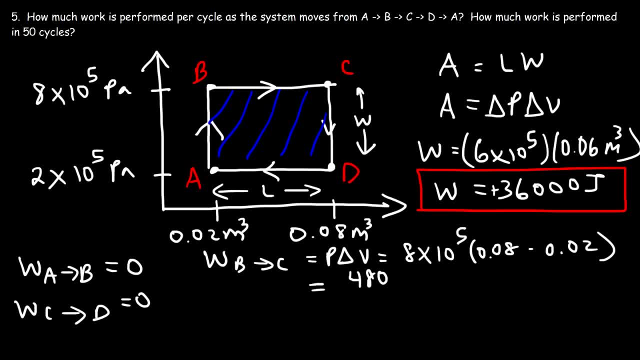 So that's equal to 48,000 joules. So we're going to have to add up these values. But before we do that, let's calculate the work that's performed, going from D to A. So the pressure at that point is 2 times 10 to. 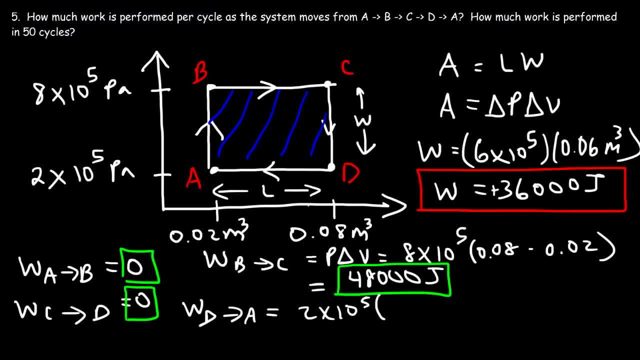 the 5. And the change in volume. the final volume from D to A is 0.02.. The initial volume is at point D, that's 0.08.. So 0.02 minus 0.08, that's negative. 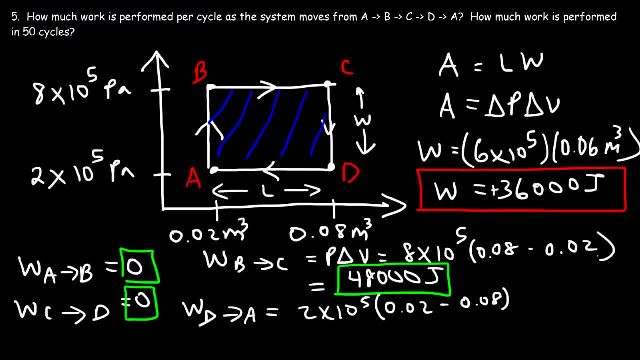 0.06 times 2 times 10 to the 5.. So this is going to be negative 12,000.. So what we need to do is add up all the values highlighted in green, So that's going to be positive 48,000. 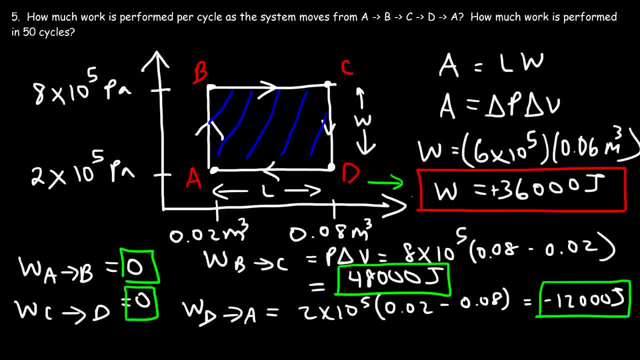 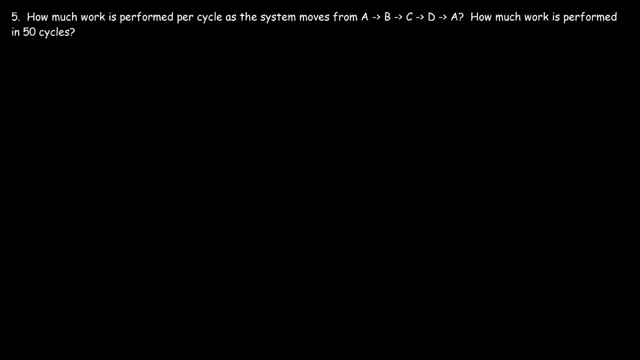 plus negative 12,000.. And that's going to give us this answer: 36,000 joules per cycle. So for one whole cycle the gas will perform 36,000 joules of work. So now, what about in 50 cycles? 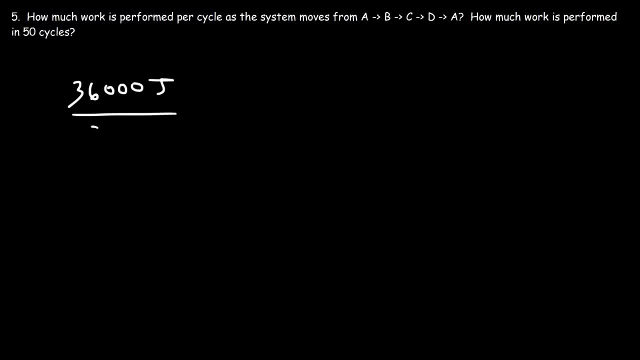 So if it's 36,000 joules for just one cycle, then all we need to do is multiply it for 50 cycles. So 36,000 times 50, that's going to be 1.8 million, or 1.8 times 10 to the 6.. So that's how much joules of. 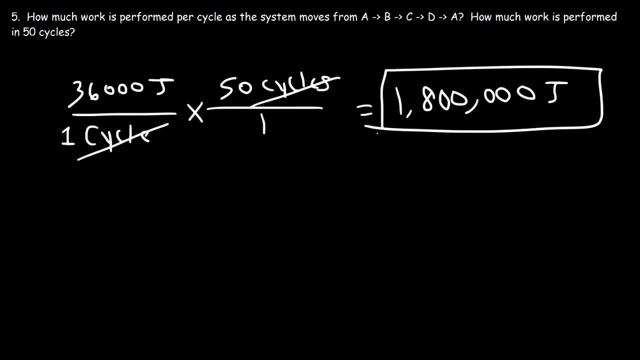 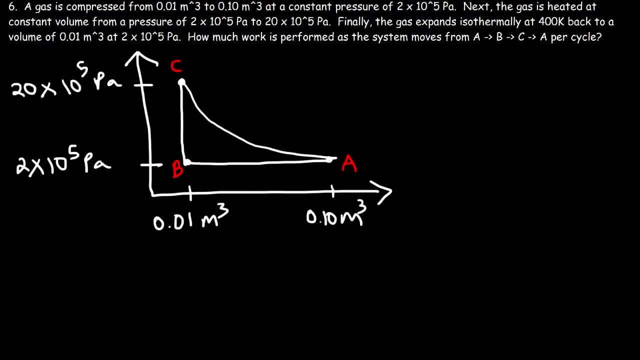 energy or joules of work, that's going to be performed over the course of 50 cycles. Now let's work on this problem. So our goal is to calculate the work performed as the system moves from A to B, and then B to C and then C to A, So from A to B. it's moving there at constant pressure, So the 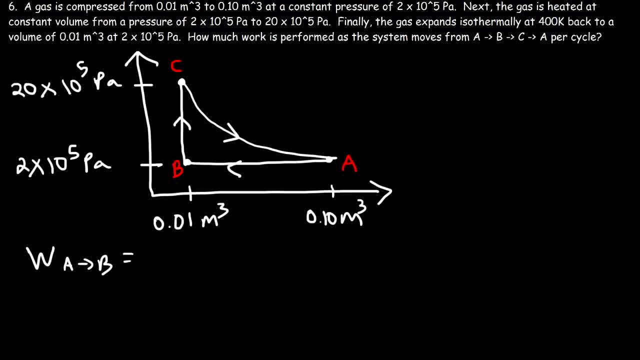 work. to go from A to B, that's going to be P delta V, And so the pressure is 2 times 10 to the 5 pascals, And then the change in volume is going to be the final volume, which is 0.01.. 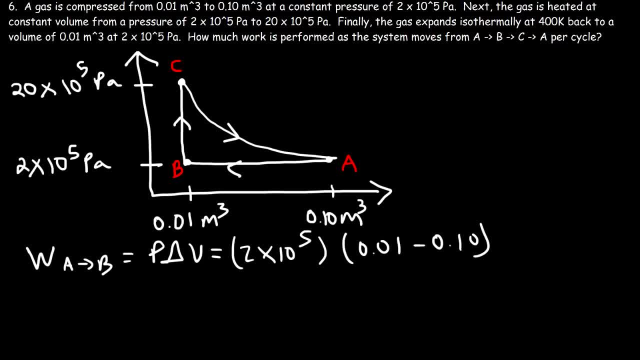 Minus the initial volume of 0.10.. So that's going to be negative 18,000 joules. Now going from B to C, we have an isochoric process. So because the change in volume is zero, the work is going to be zero for that process. 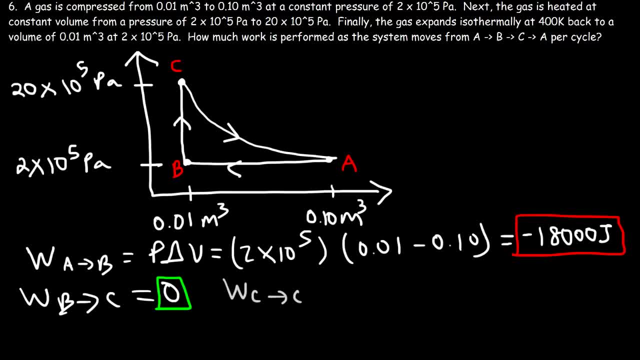 Now from C to A, it expands isothermally. So therefore we can use this equation: nRT times ln, V final divided by V initial. And the one thing I forgot to do is give you the number of moles of gas. So let's say the number of moles is 5.. That's not going to affect. 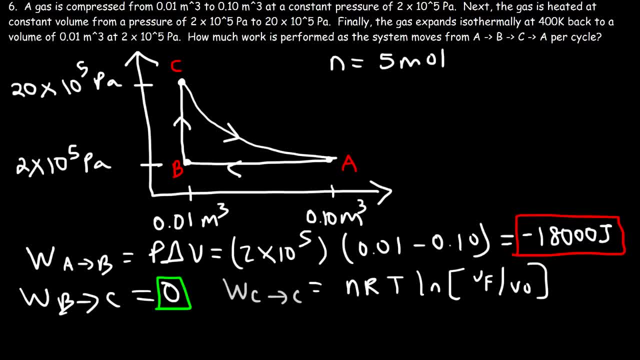 this answer Subtitles by the Amaraorg community, Or actually, you know what? We can calculate the number of moles, So turns out that I really didn't need to give you it, So we can use this equation: PV is equal to nRT. Now 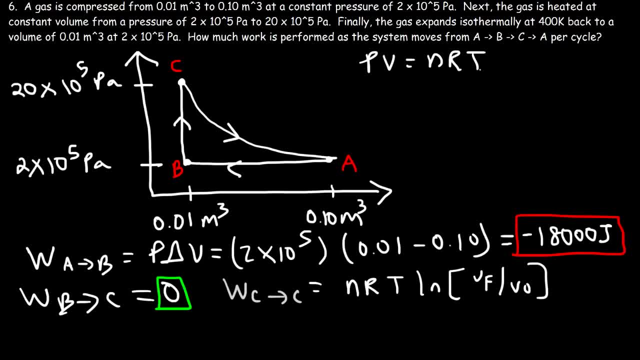 the pressure at. we need to choose a point. So, going from C to A, the temperature is held constant, So we can use point C or point A. I'm going to use point C, So at point C I'm going to use 0.05.. 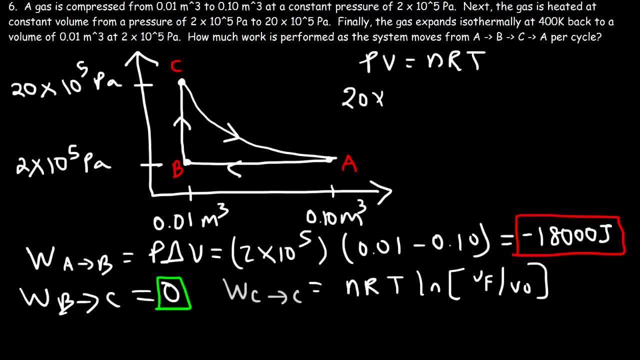 At point C the pressure is 20 times 10 to the 5 pascals and the volume is 0.01 cubic meters. Our goal is to calculate N, and R is going to be 8.3145 if the pressure is in pascals. 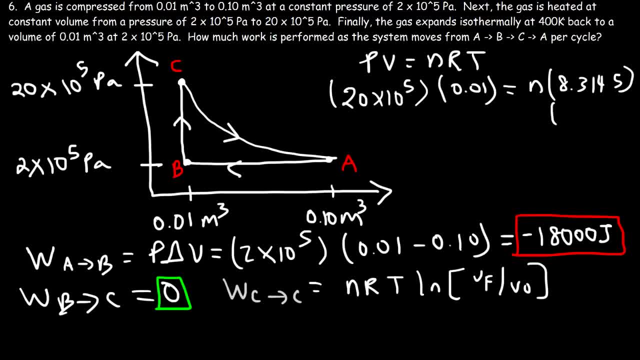 and if the volume is in cubic meters and the temperature is 400 Kelvin, So it's going to be 20 times 10 to the 5, multiplied by 0.01, that's 20,000.. Divide that by 400, and then divide that by 8.3145.. 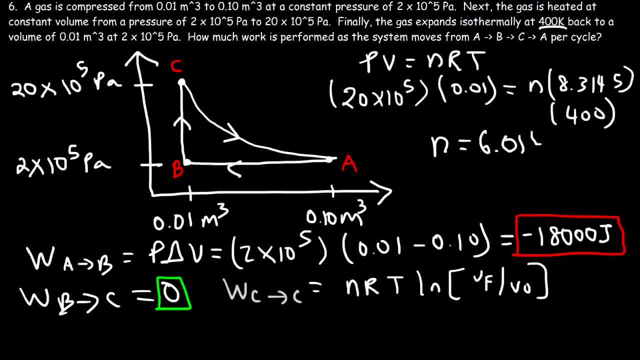 So N is 6.014 moles. So now we could use this formula to calculate the work going from C to A. So it's going to be N, which is 6.014, times R. Okay, That's 8.3145, multiplied by the temperature, which is 400 Kelvin in this example, and then 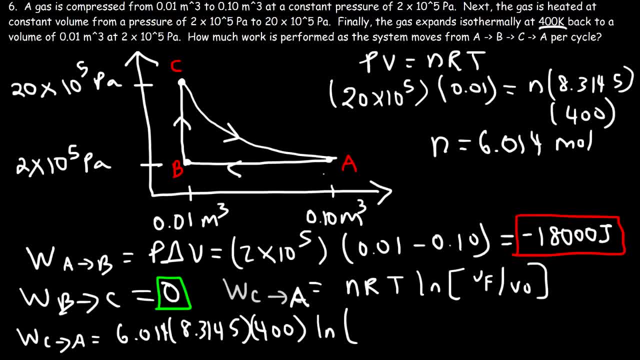 times LN. Now, going from C to A, the volume changes from 0.01 to 0.10.. So the final volume is 0.10, and the initial volume is 0.01.. So go ahead and type this in. 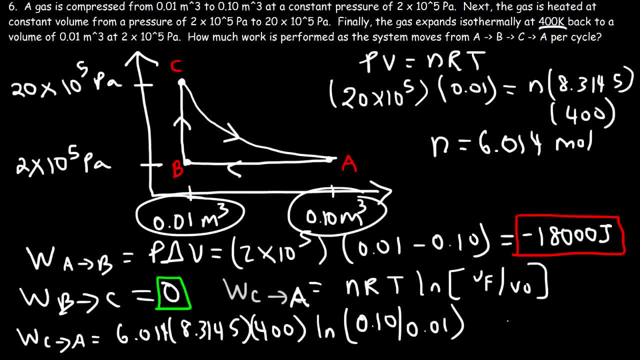 So this is going to equal 46,055 joules. So the total work is going to be the sum of these three highlighted values. So it's going to be negative 18,000 plus 46,055.. So that's going to be positive 28,000. 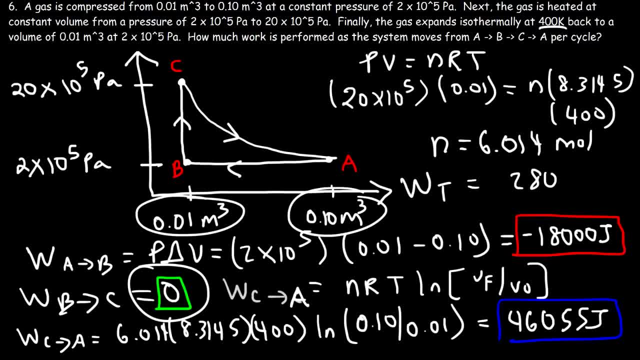 So that's going to be positive 28,000.. Okay, So that's going to be positive 28,055 joules. So that's the answer And we can see why the network done is positive. As we mentioned before, the system is moving in this direction, in the clockwise direction. 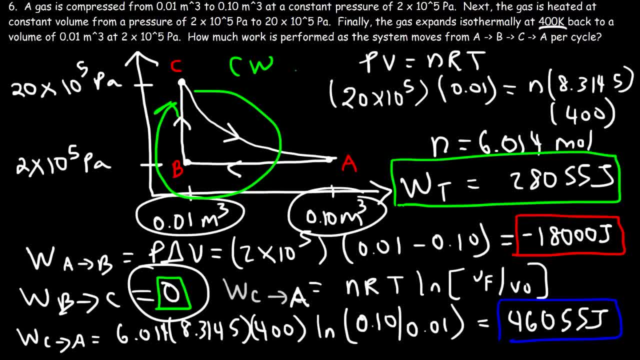 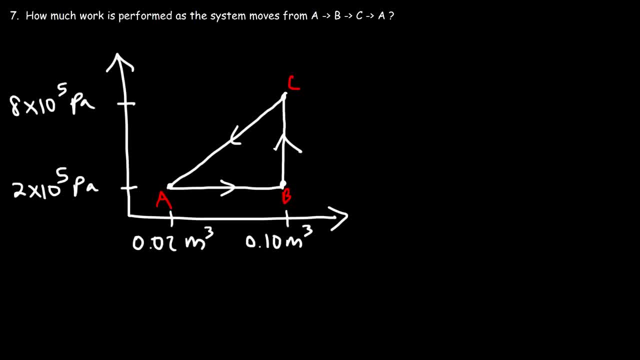 If it was going counterclockwise, the network done would be negative as opposed to positive. Number seven: how much work is performed as the system moves from A to B to C and back to A. So for a cyclic process, we just got to find the area enclosed by this PV diagram. 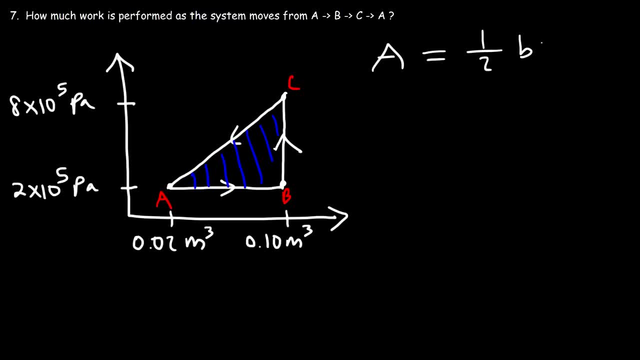 So we have a shape of a triangle and the area of a right triangle is one half. based on site, The base is the change in volume. So the change in volume 0.10 minus 0.02, that's 0.08.. 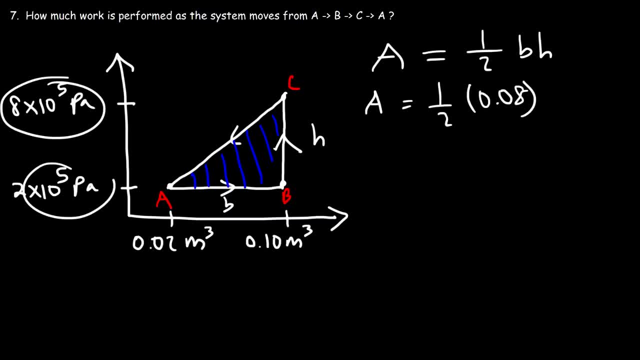 And the height is basically the difference in pressure. So 8 minus 2, that's going to be 6.. Half of 0.08 is 0.04 times 6 times 10 to the 5. So the work is going to be 24,000 joules. 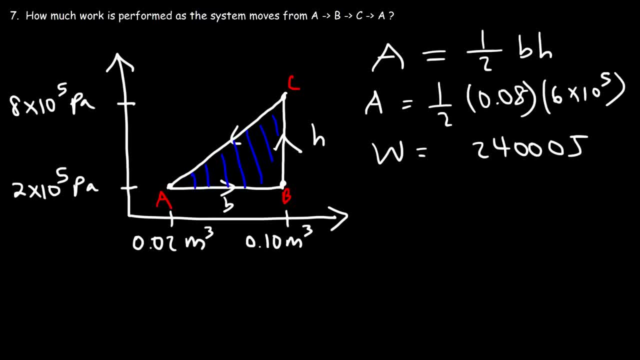 Now, is the cycle clockwise or counterclockwise? Notice that it's going in this general direction, So that's counterclockwise. Therefore, the work done should be negative as opposed to positive. So the work done per cycle is negative. 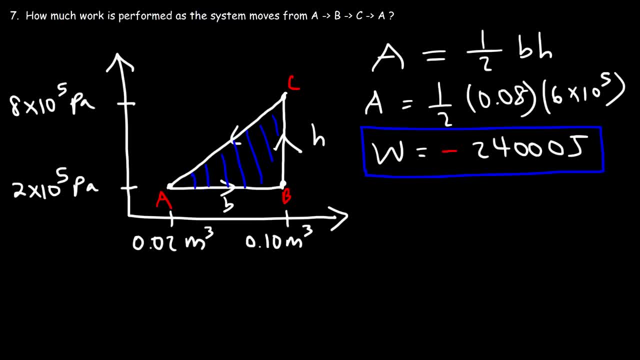 So the work done per cycle is negative 24,000 joules. Now let's confirm this answer by calculating the work done for every segment. So let's start with A to B. Going from A to B, that's an isobaric process. 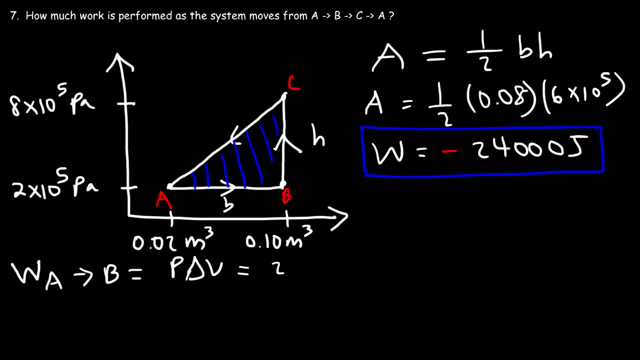 So it's simply pressure times the change in volume. So the pressure is 2 times 10 to the 5 pascals, The change in volume is going to be the final volume, 0.10, minus the initial volume of 0.02.. 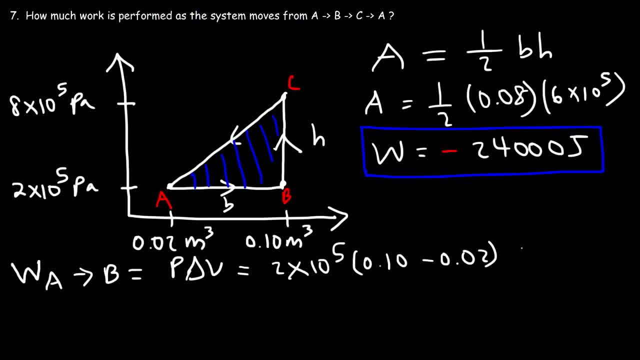 So 0.10 minus 0.02, that's 0.08, times 2 times 10 to the 5.. So this is going to be positive 16,000 joules. Now let's calculate the work going from B to C. So that's an isochoric process. 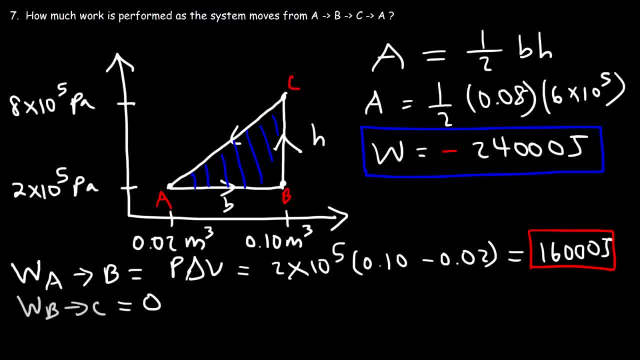 The volume doesn't change, So the work there is going to be 0.. Now what about going from C to A? What can we do? In going from C to A, notice that it's a straight line. The volume is changing and the pressure is changing. 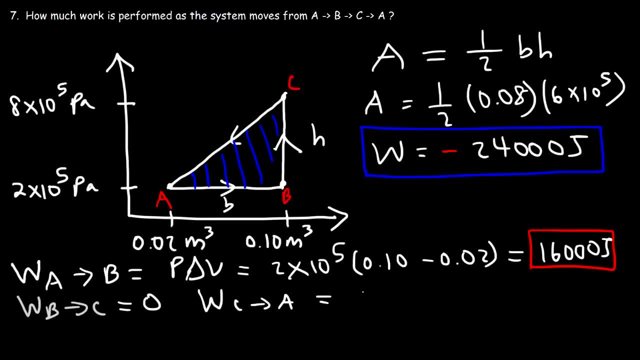 So it's going to be very similar to this equation, but it's going to be an average pressure, So it's going to be 1 half times the initial plus the final pressure multiplied by the change in volume. So the initial pressure going from C to A, That's 0.10.. 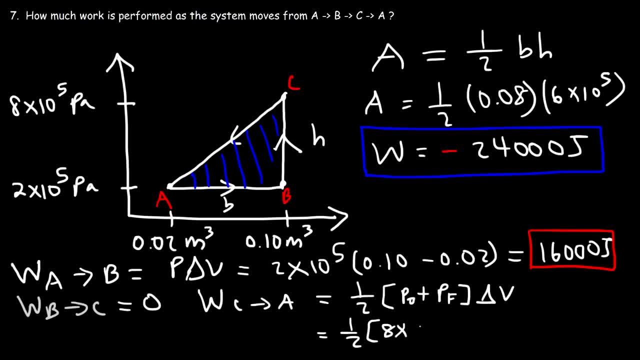 What can we do? So we're going to be 1 half times the initial plus the final pressure multiplied by the change in volume, That's 8 times 10 to the 5.. The final pressure at A is going to be 2 times 10 to the 5.. 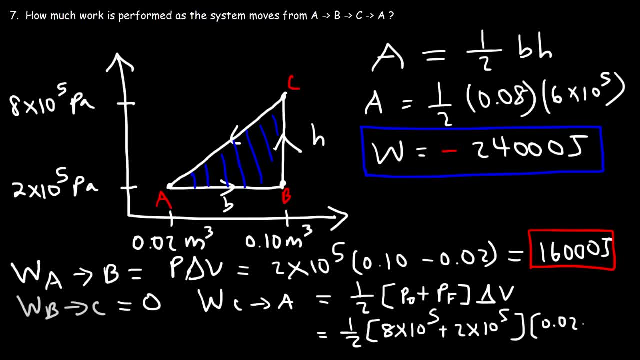 And the change in volume. the final volume is 0.02, the initial volume is 0.10.. Let's see if I can fit that here. So 8 plus 2 is 10.. One half of 10 is 5..